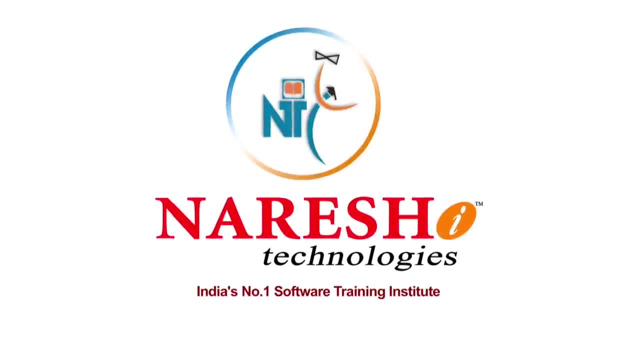 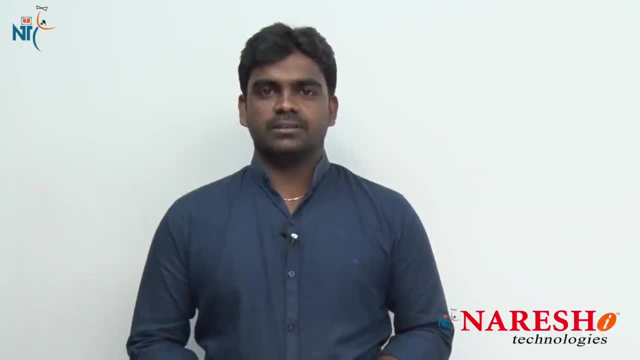 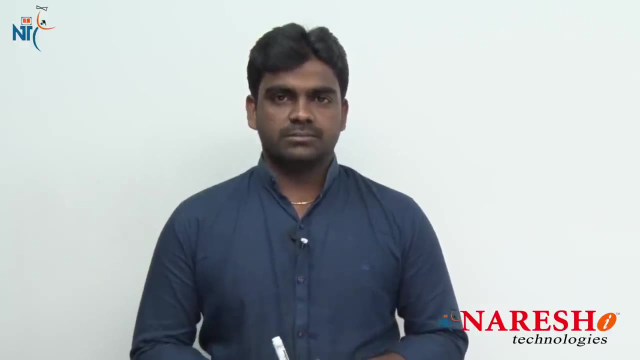 Welcome to Naresh Technologies. this is Srinivas. So in the last session so we had discussed so what is a variable and what is a function? So these two are the main building blocks to develop application, so to write a program. Now we will see how many classifications 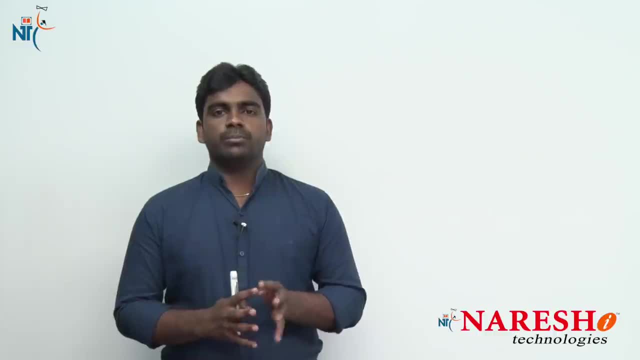 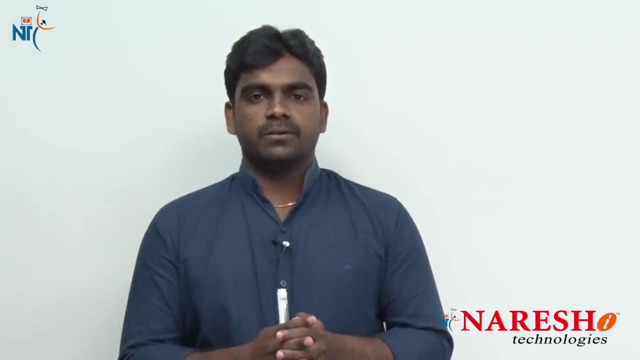 right of a method. So generally only four method classifications are present. So whatever the programming language you take- So this is not only for C language- C, C plus plus, Java, dot net, wherever you go Any text book, you open all right, any program, you see, If 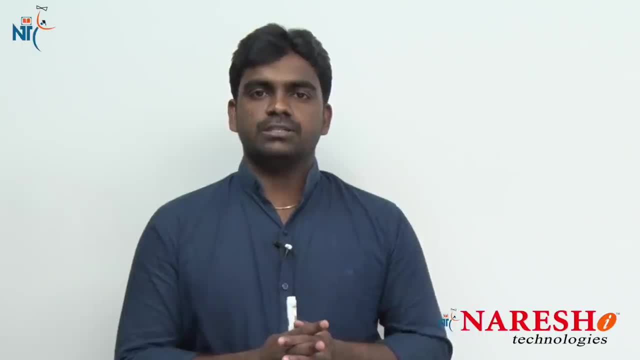 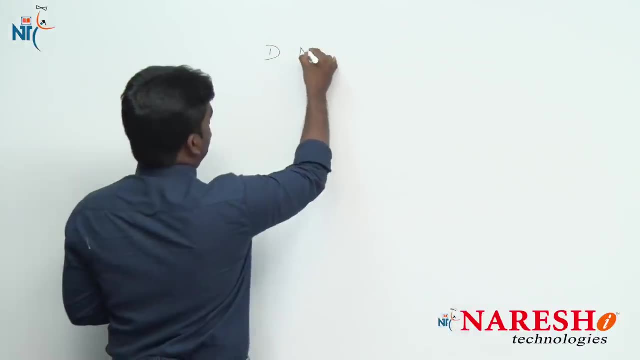 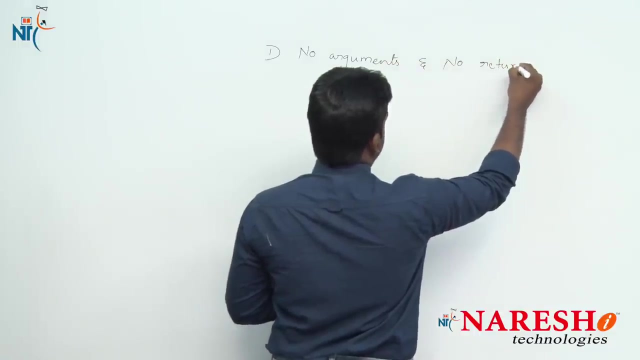 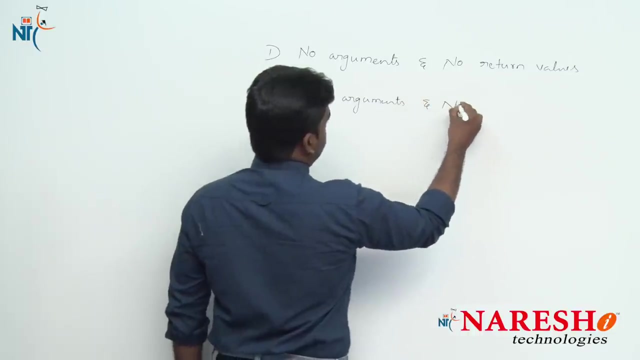 you look at one particular method or one particular function, the function belongs to any one of these four classifications. The first one: no arguments, no arguments and no written values function. Second one: with arguments and no written values function. Third one: with arguments and no written values function. 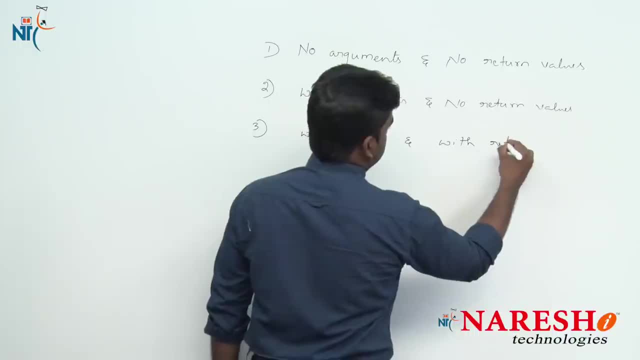 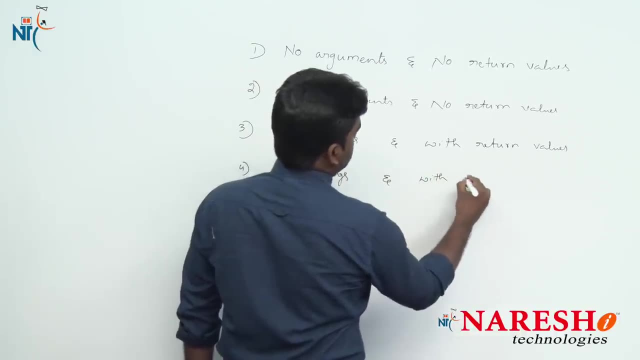 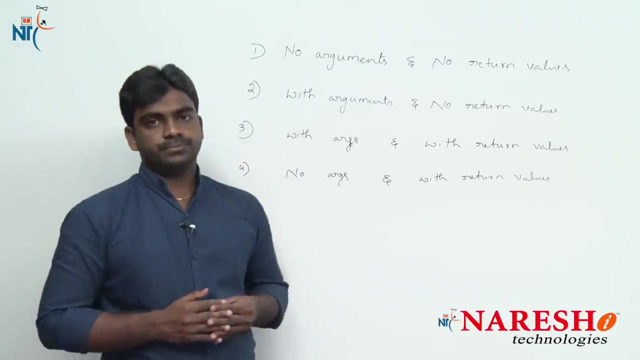 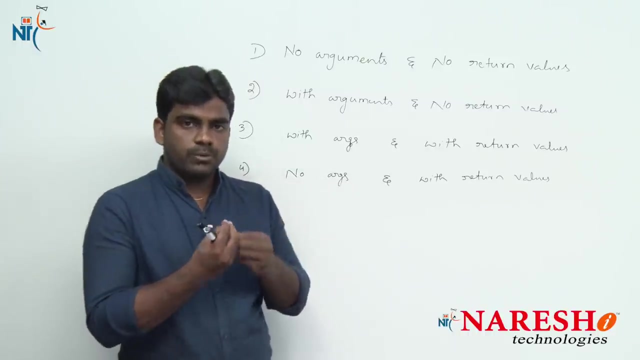 And the last one: no arguments and with written values, function. These are the four classifications available for a method. So before so discussing all these four classifications, So first we need to remember once again what is a function. A function is a set of instructions. 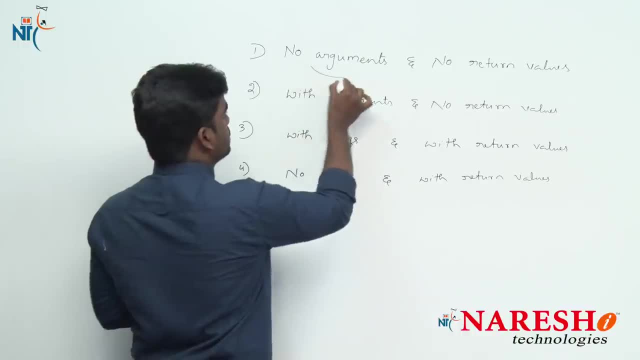 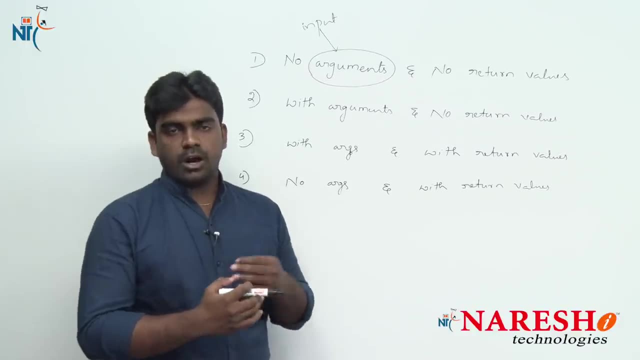 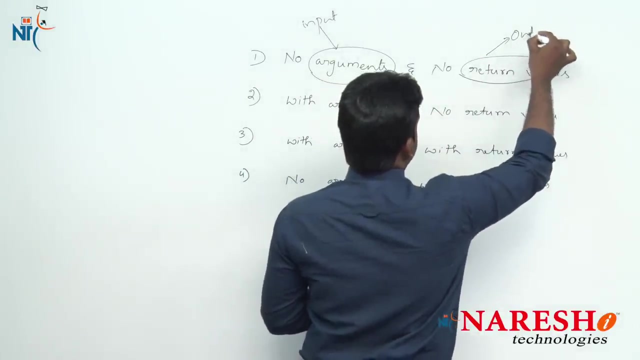 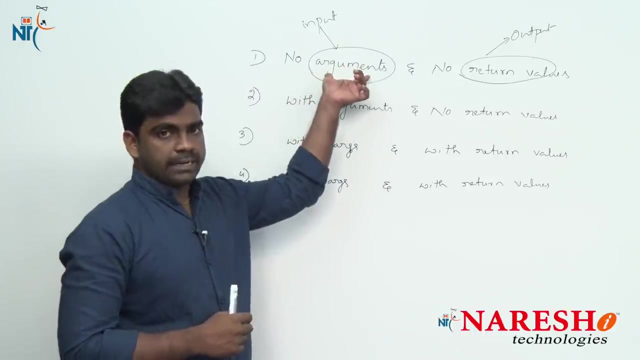 it is taking input. arguments is called input. arguments is called input. After processing the input, after processing the information right, it will produce that output, that return value. we can call it as a output. A function is a block of instructions- is taking input. 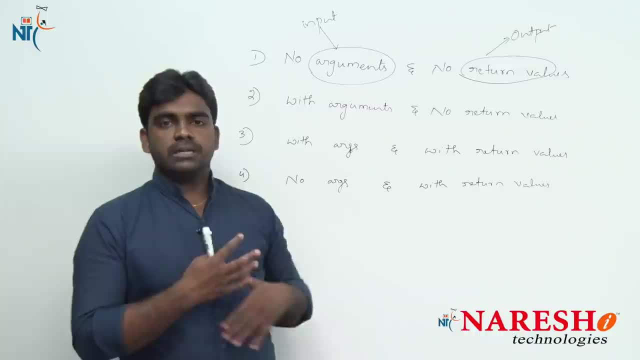 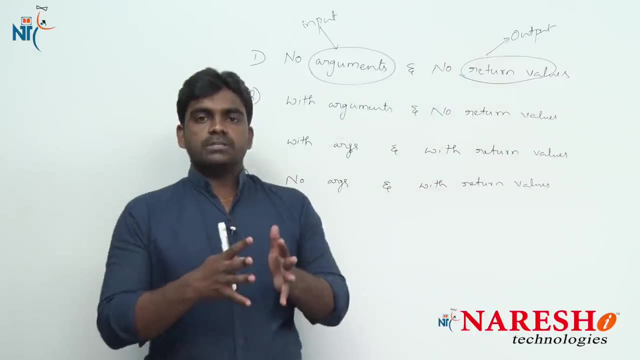 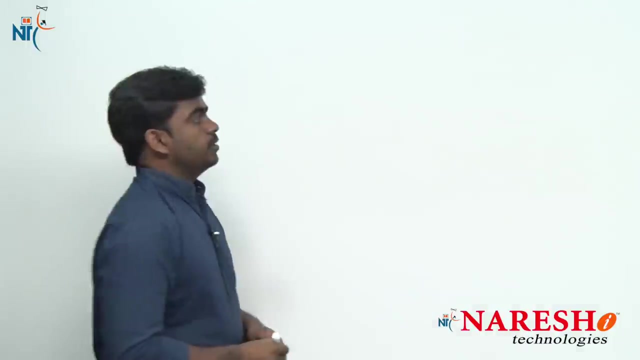 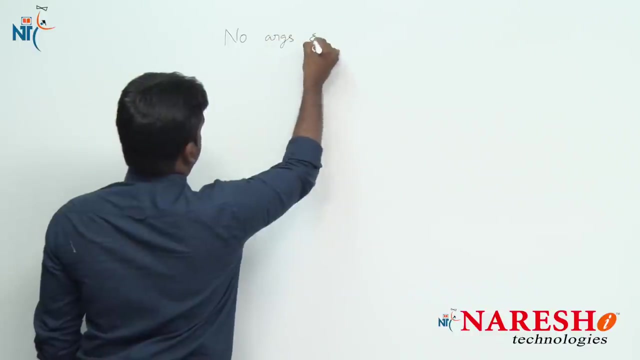 technically arguments and after that it is processing that input using the predefined. after processing it will produce that output. So depends on the method, syntax only. So now we will discuss all these four classifications. ok, See four classifications here. the first one: we are writing no args and no return values. 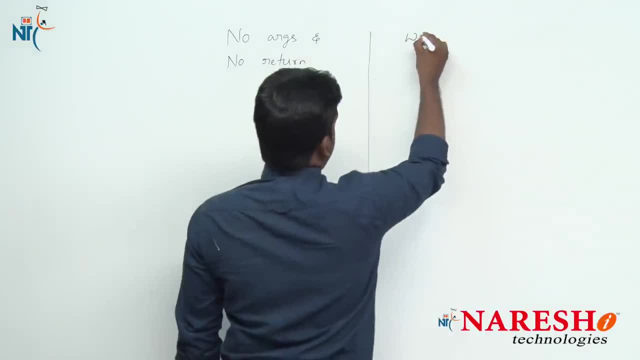 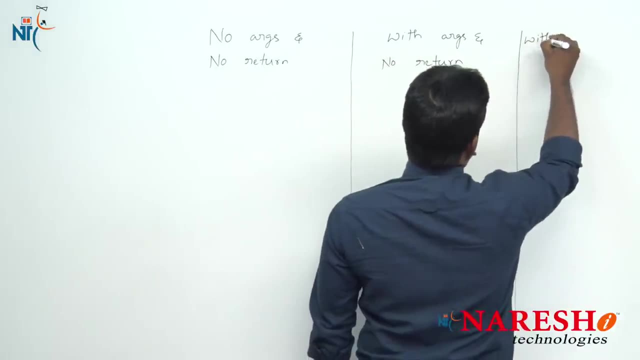 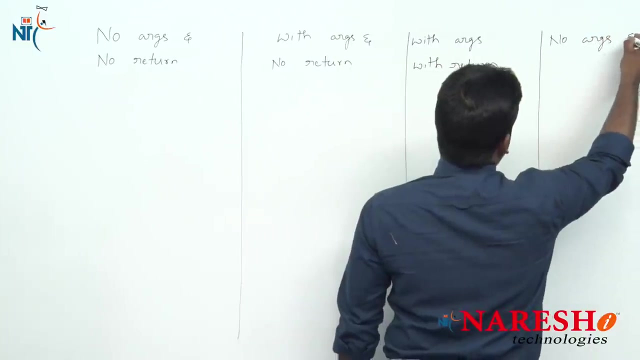 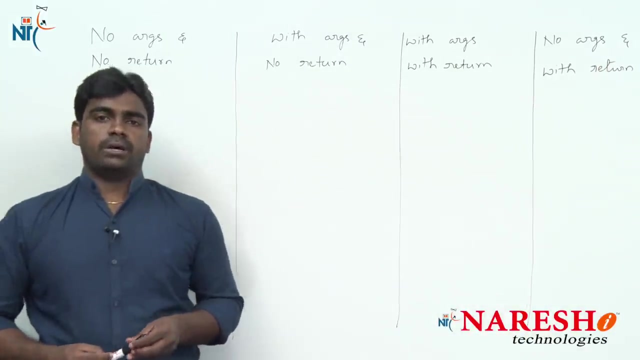 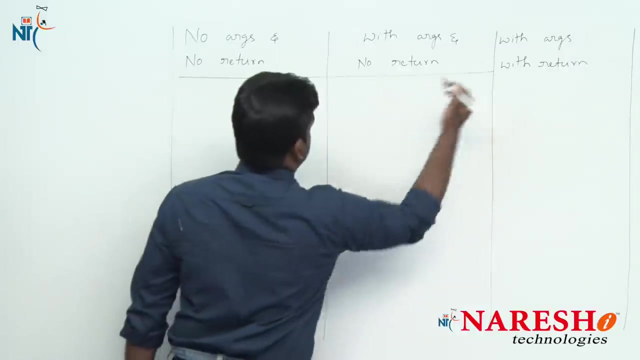 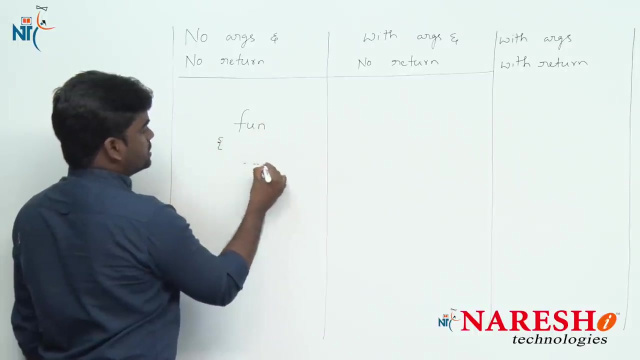 is a first classification. second one with args and no return values, third one with args, with return values and the last one, no args and with return values, no args and with return values. see that classification: First classification: no args and no return values. I am writing one function, just function name. I am taking fun. it is a block of instructions. 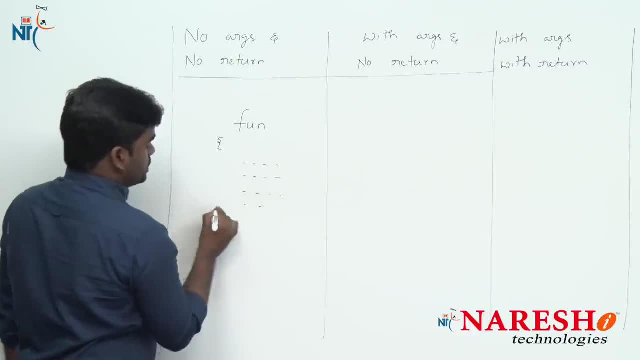 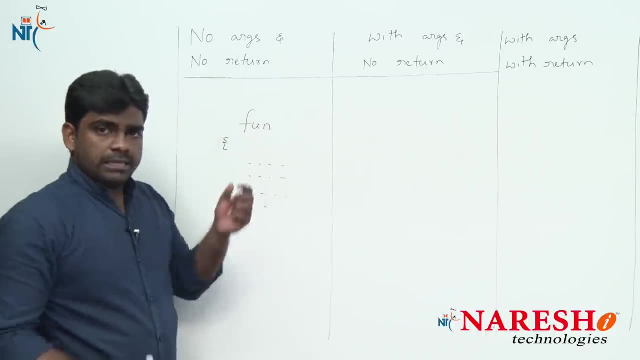 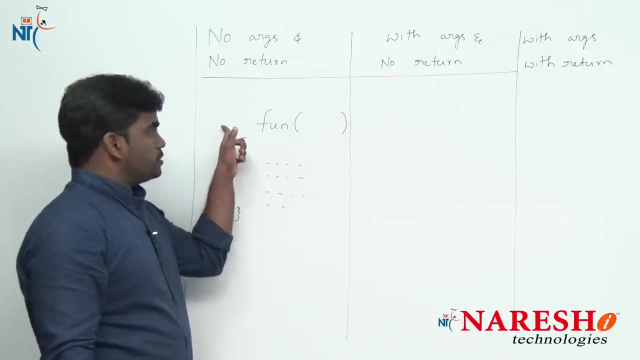 we already discussed. here you will write the logic, the function logic we need to place inside this block. any logic you can write The function is taking input is nothing but arguments. here it is. this is arguments place and this is a return values place. but here, 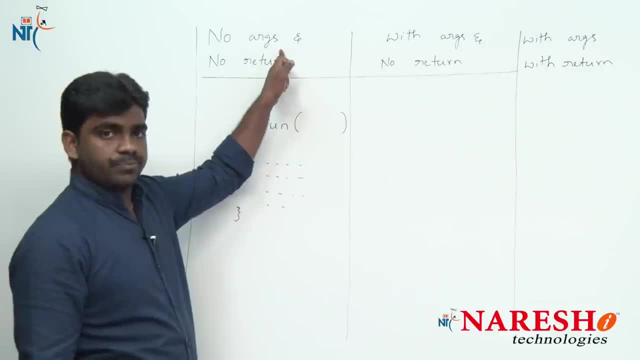 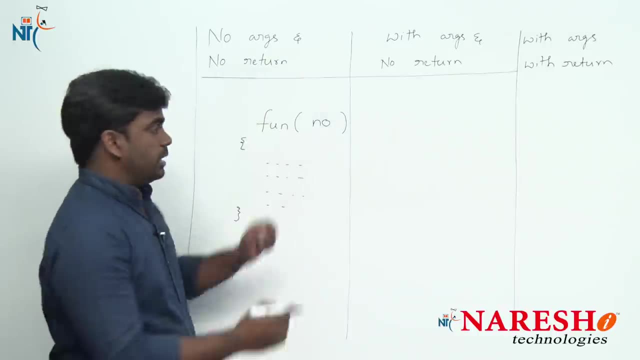 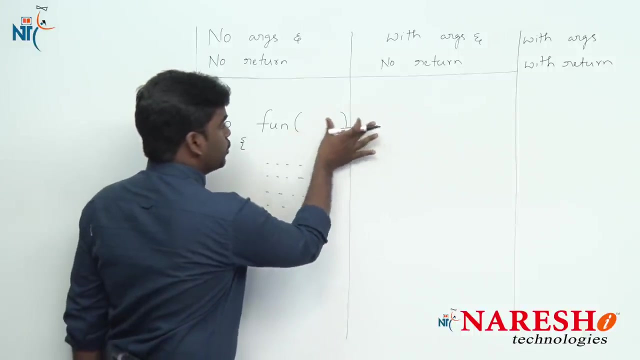 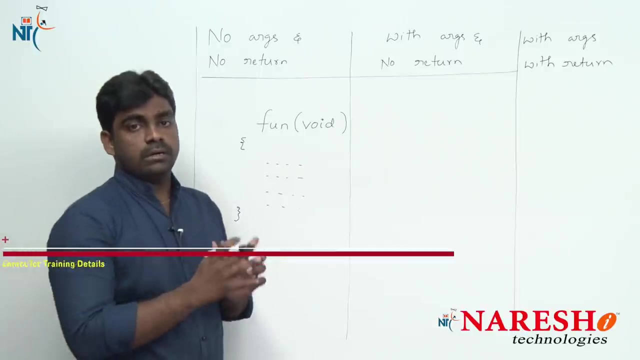 it is. what is our classification? No arguments. so here it is. we need to write a no arguments and no return values, and here also we are writing no. but here it is, instead of writing no. they have given one technical keyword in programming languages is called void. void is representing no, nothing. So 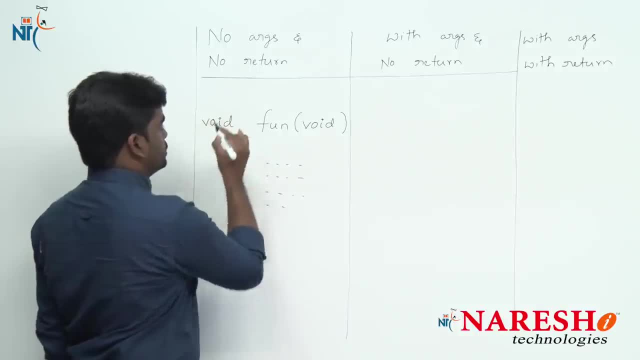 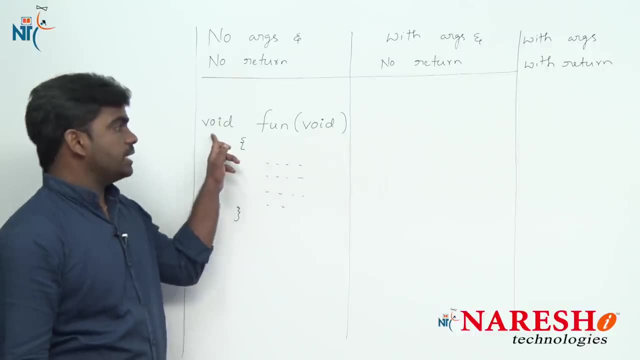 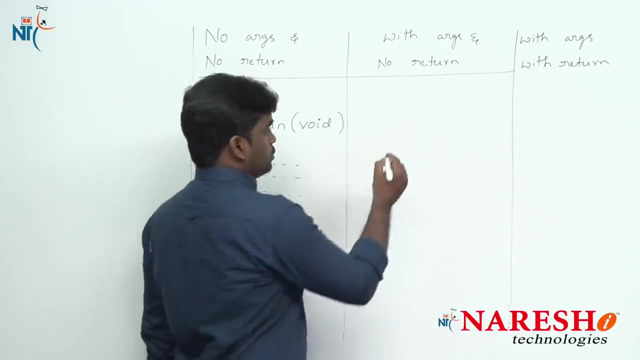 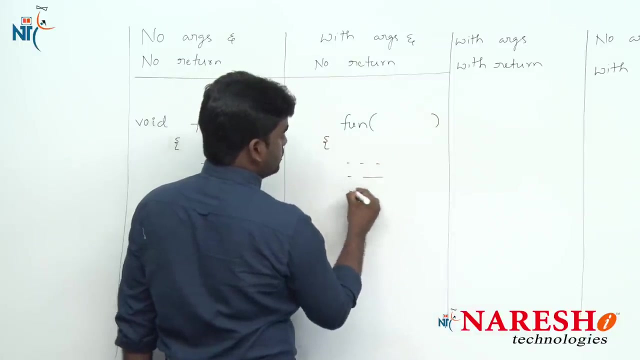 no arguments and no return values: function. So function is a block of instructions, is not taking any arguments and not returning anything to anyone. Next come to that second classification with arguments: no return values. So function with arguments. we need to pass some arguments. we need to pass arguments. 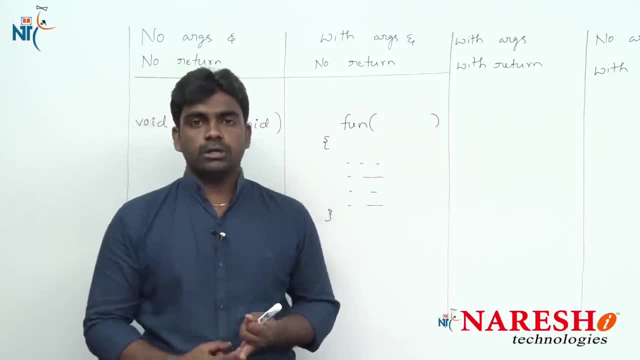 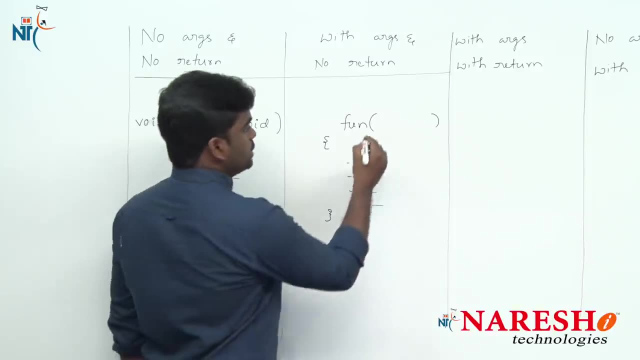 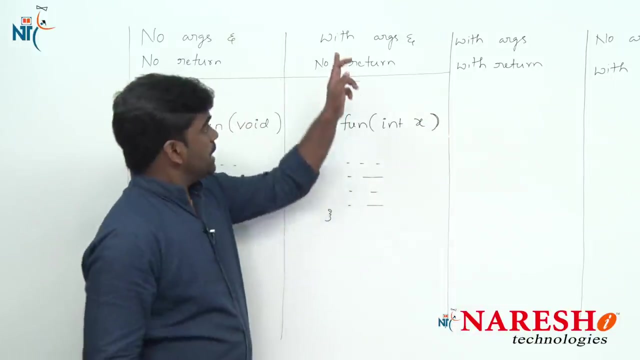 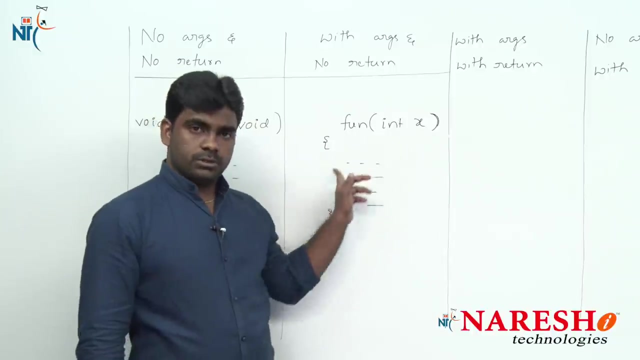 Sir, what are the arguments? some values, integers, float, double character strings- all these are comes under input types. Simply, I am passing only one integer to collect that we are declaring one variable. this is called arguments. Look at the classification once with arguments. so we need to pass arguments and next it will process that input with the predefined logic. 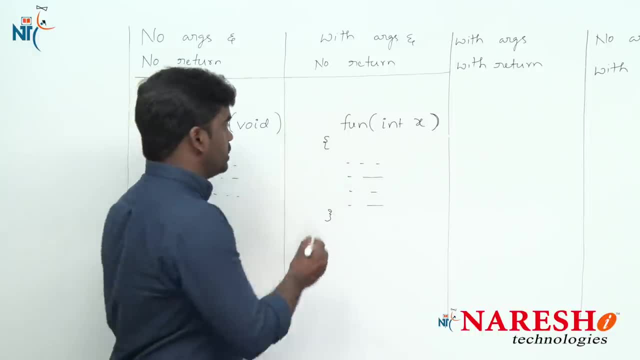 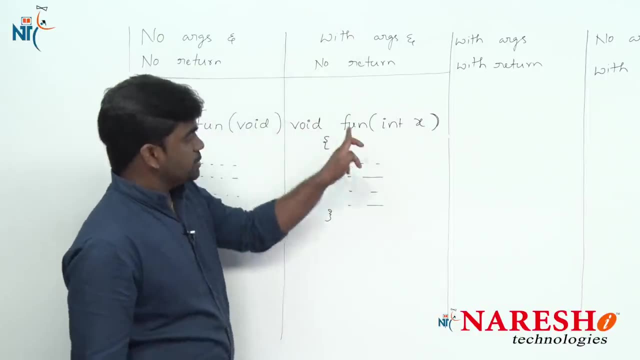 and finally it will return the output. Output is a void because no return values. look at the classification. So the function is taking arguments with arguments, but it is not returning anything. no return values is the classification, second classification. Now come to the third classification. 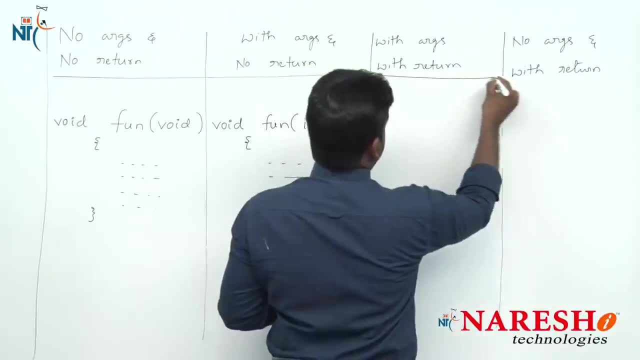 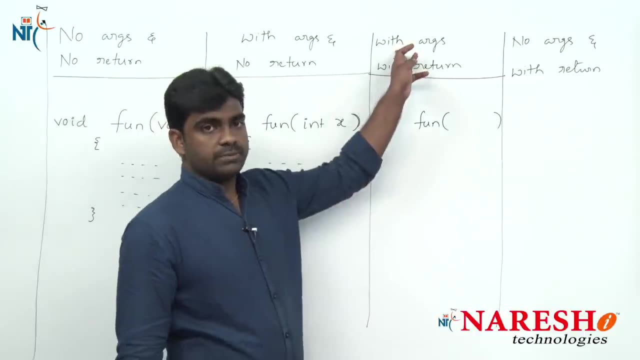 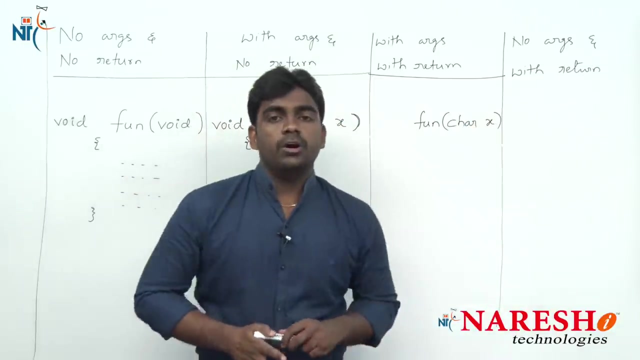 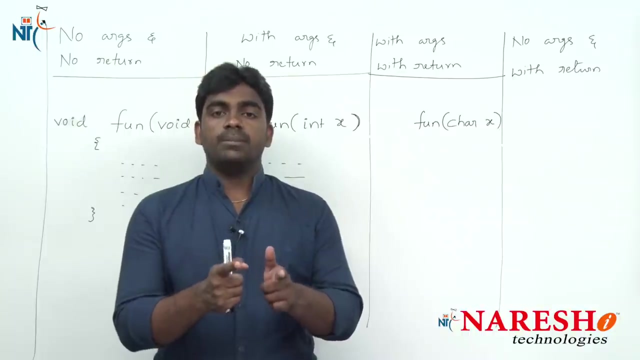 with arguments and with return values. classification Function is taking arguments with arguments. here it is suppose we are passing character. any arguments we can pass, Sir. how many arguments we can pass? no limitations, hundreds of hundreds of arguments we can pass- depends on your application requirement. 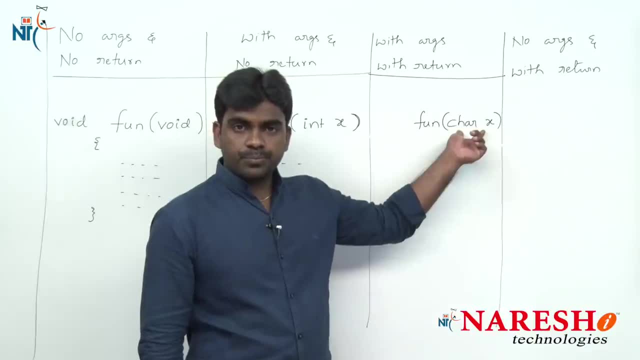 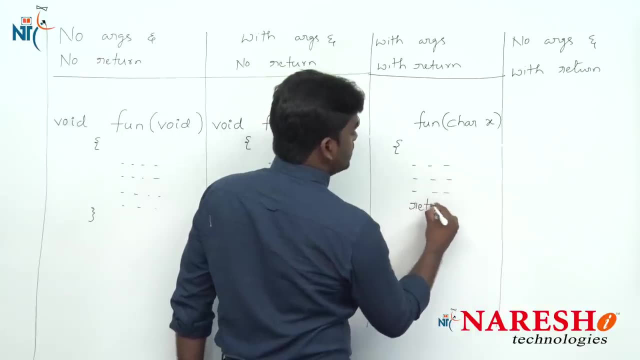 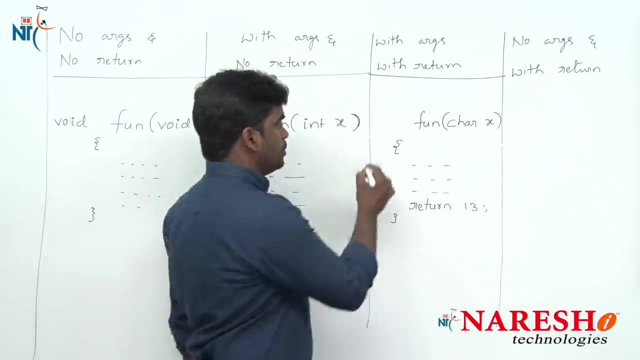 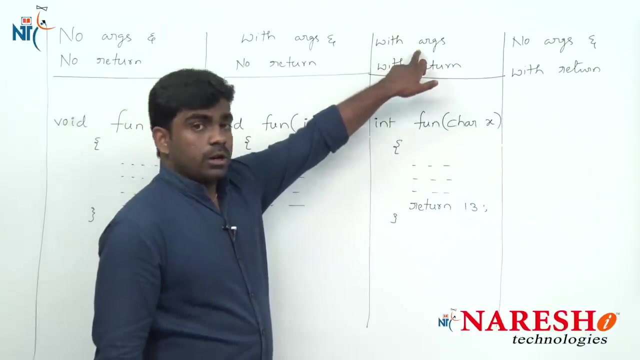 So here it is. simply I am passing only one argument character and here with return values, So return statement mandatory. suppose I am returning 13,. 13 is of type. what is an integer type? So return type is a integer. the function with arguments. 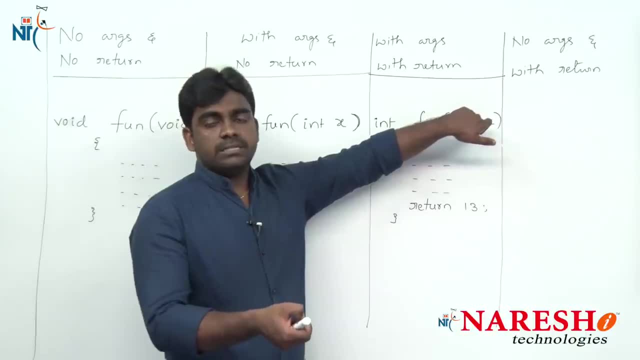 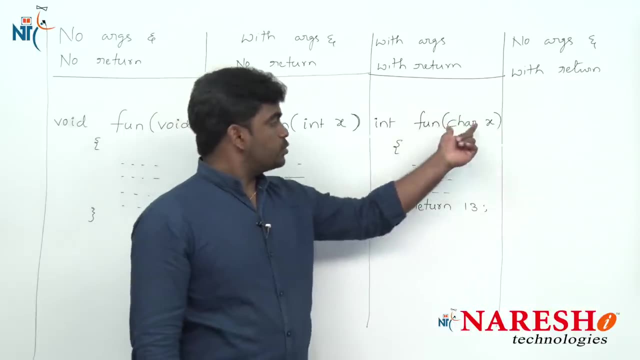 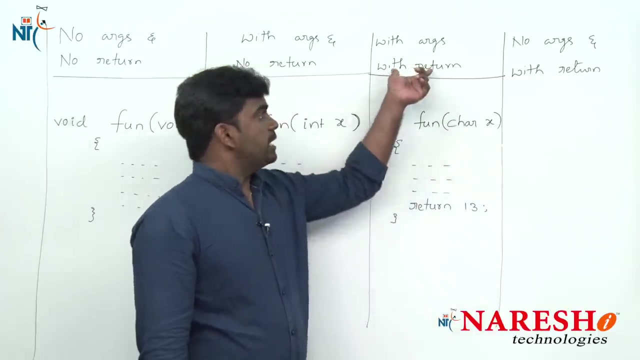 So here it is taking arguments. what type arguments it is taking, no matter. first it is taking arguments or not, that we have to consider. So here it is taking arguments. and next what it is returning? integer data. it is returning with return values means return statement is compulsory. it is mandatory to define. 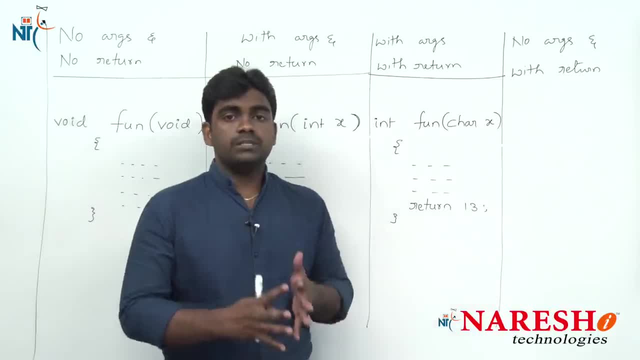 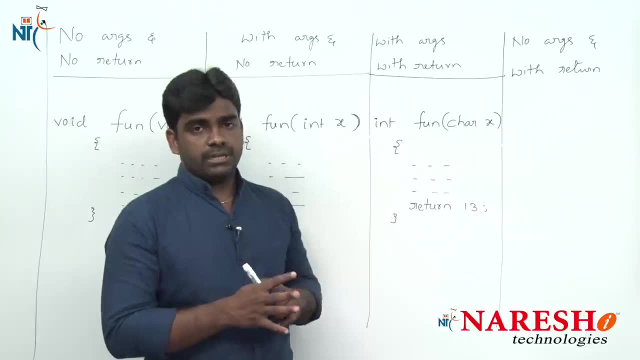 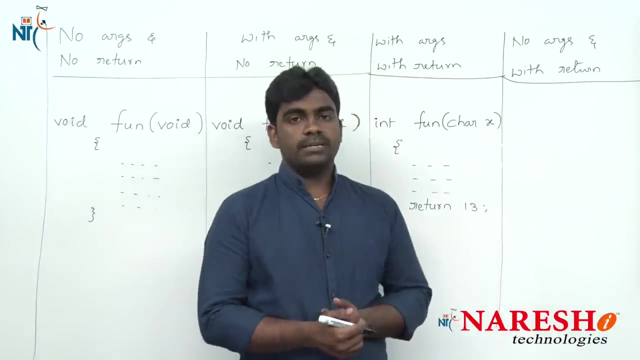 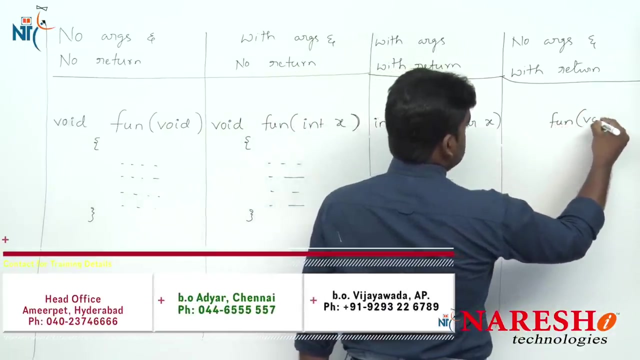 So return statement 13 it is returning. 13 is of what type of data? integer data. So return type is also integer. and next the last classification: no arguments and with return values. no arguments and with return values: See here now fun. no arguments means void. we need to write. 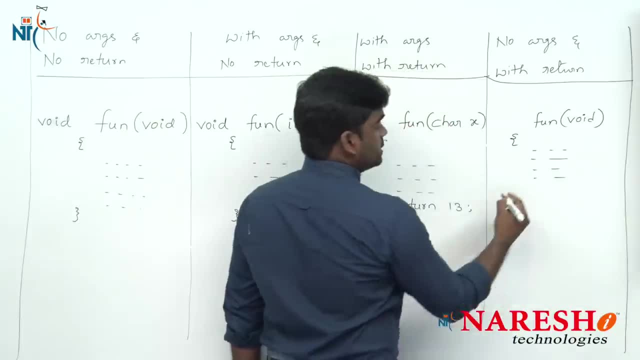 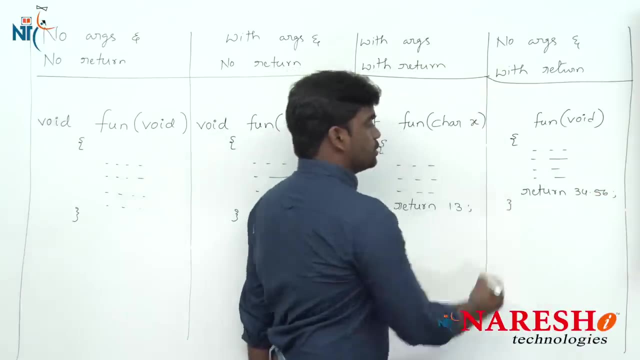 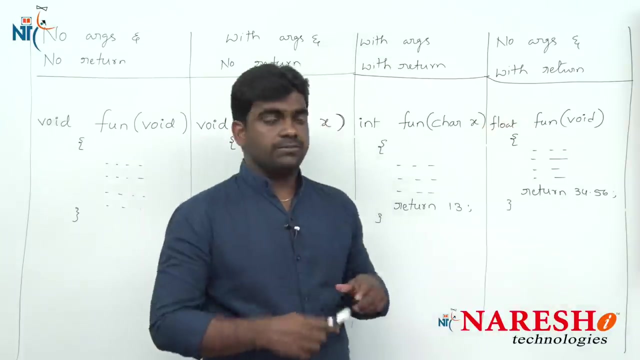 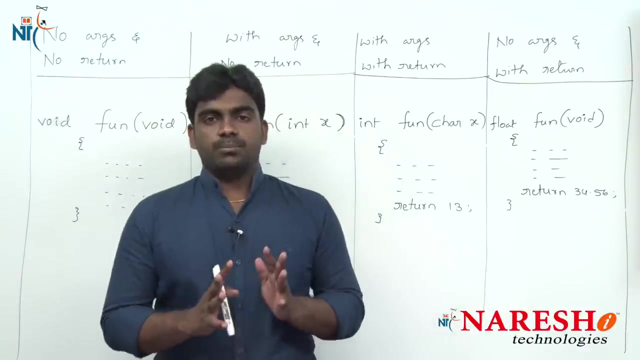 Void With, With return values, what it is returning. suppose here it is returning the value 34.56, 34.56 is of type, float type or double type. So here it is a return type is also float type. So classification: no arguments and with return values only four classifications are present. 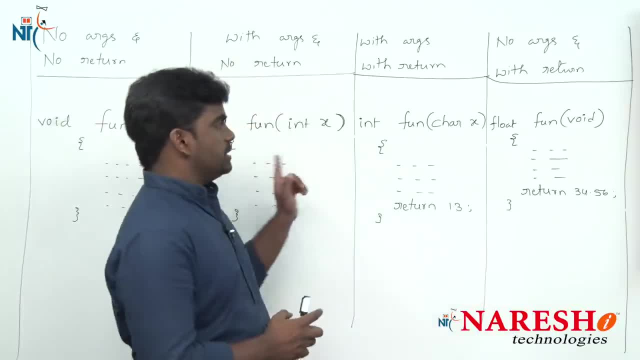 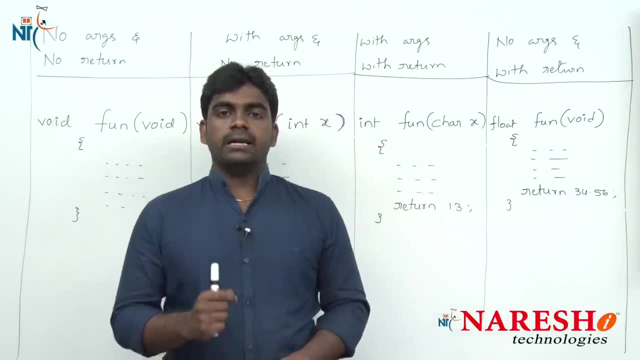 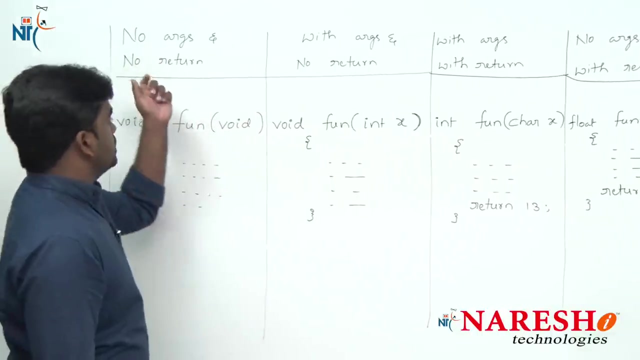 for a function or method. these four classifications very easy to understand In every program, from day one to day end, right in every program we always define any one of these four methods only in any programming language. So that much important four classifications clearly we can understand. first one is a function. 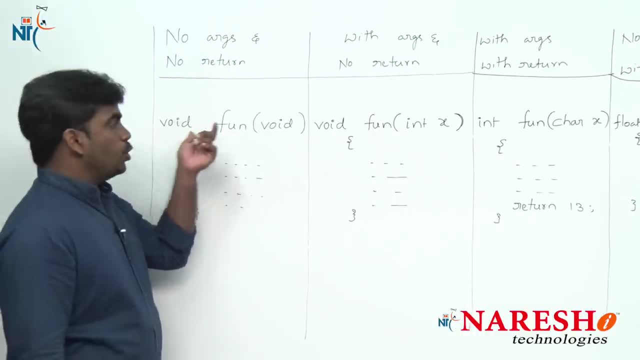 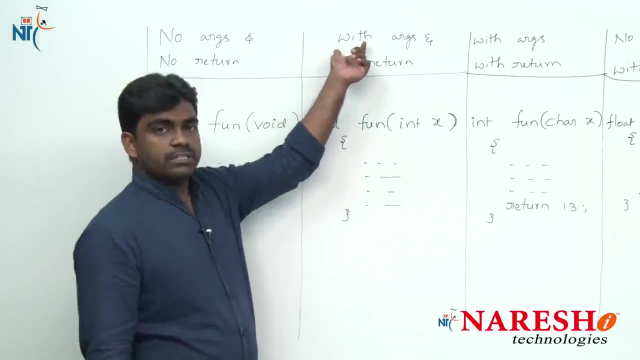 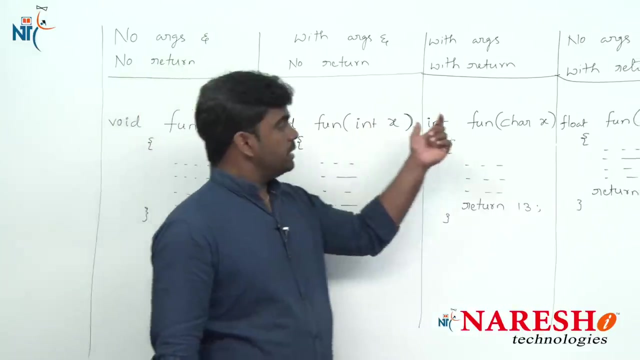 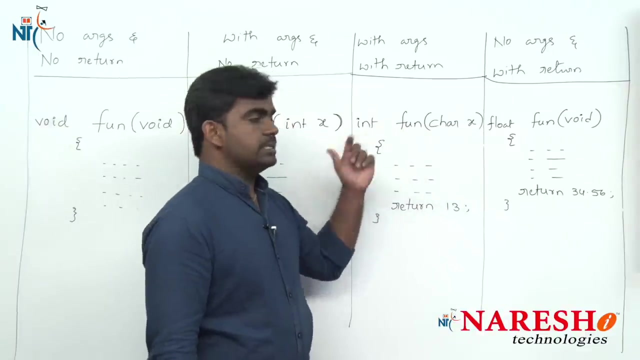 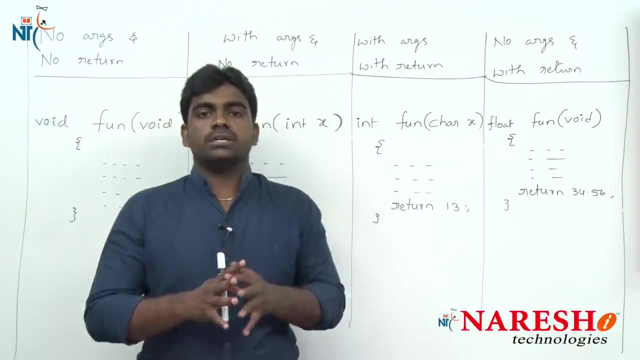 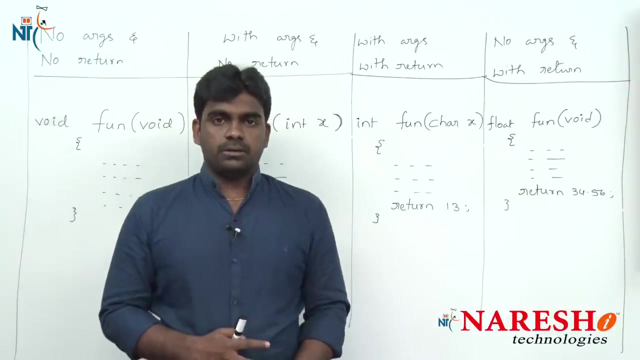 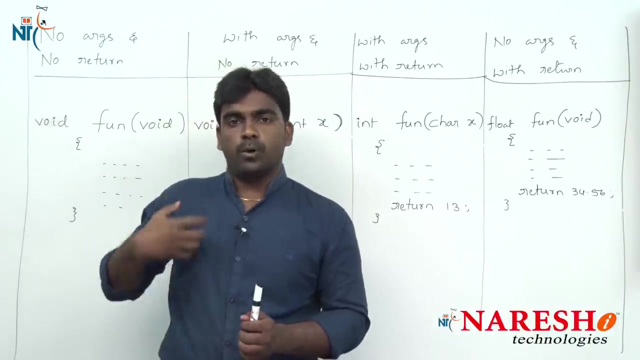 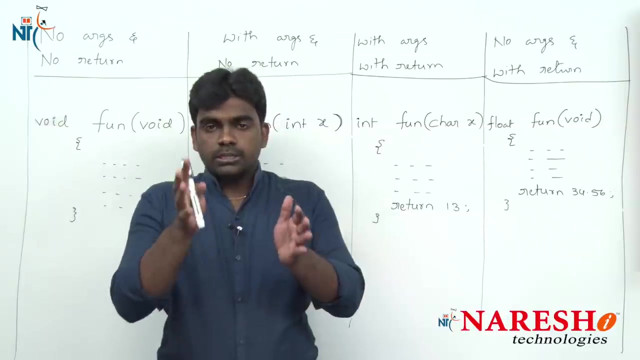 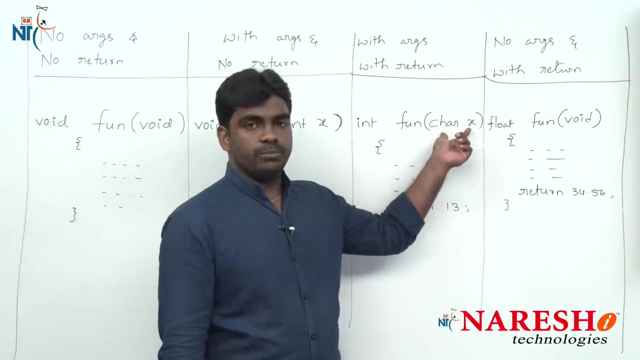 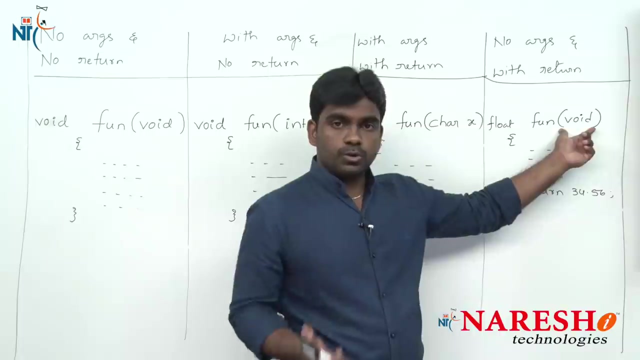 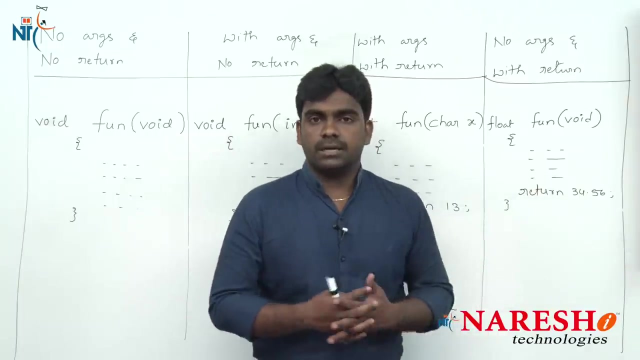 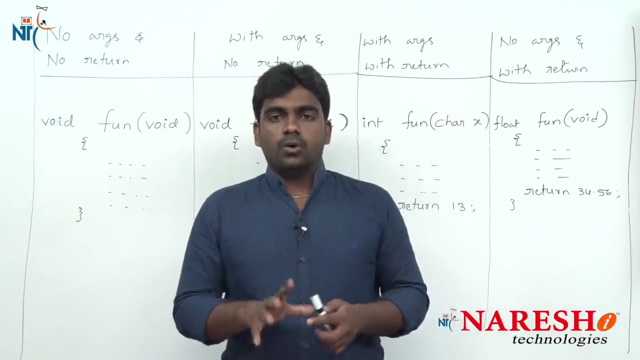 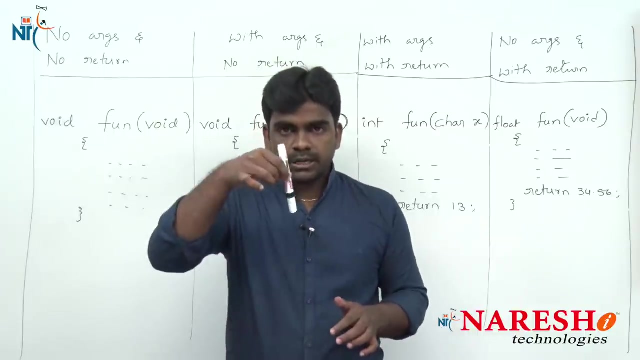 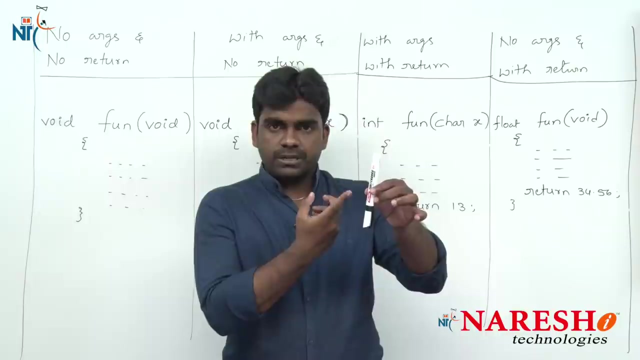 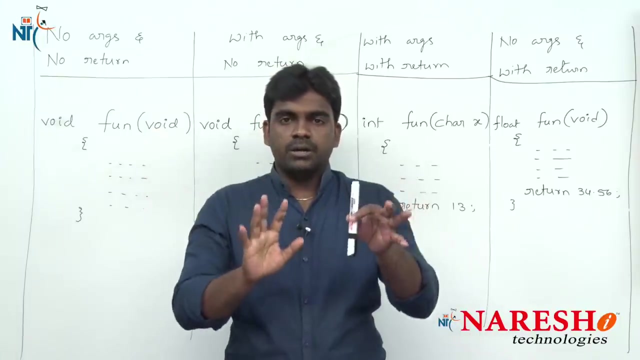 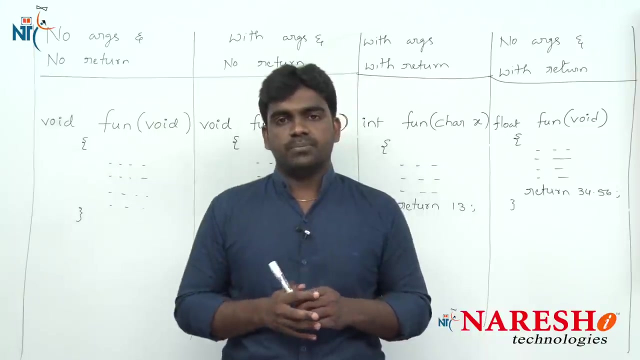 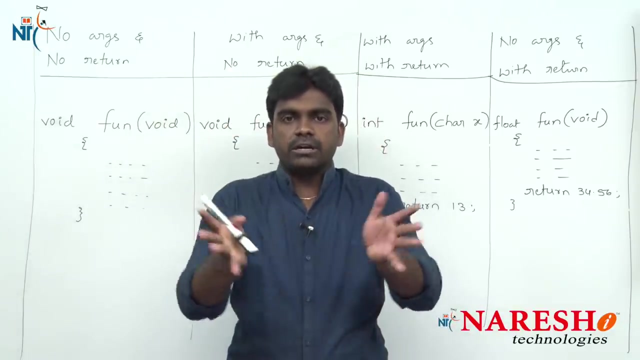 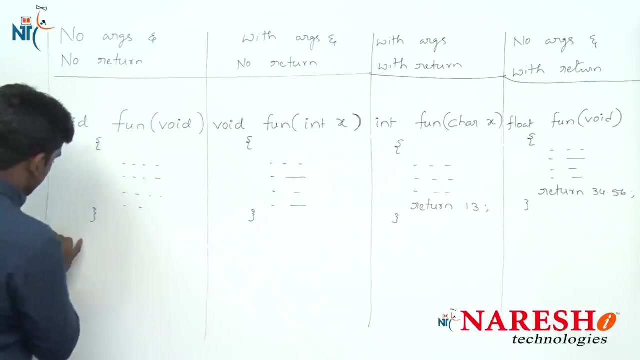 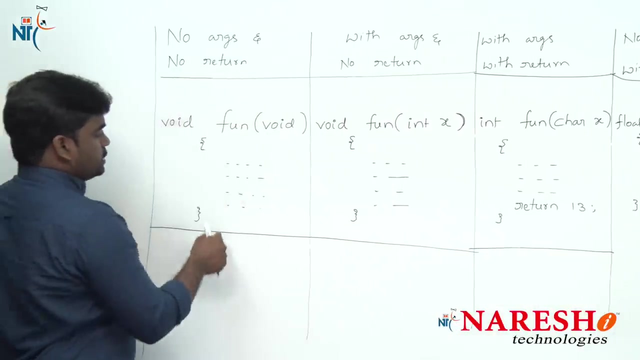 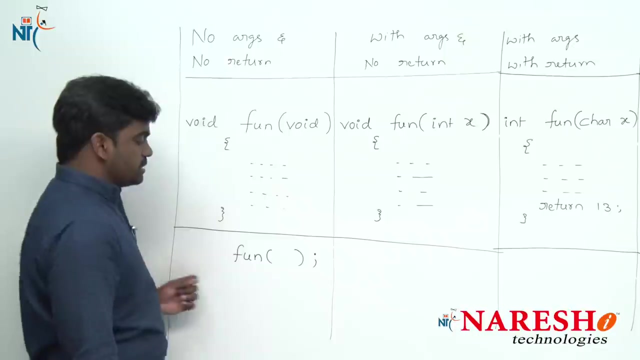 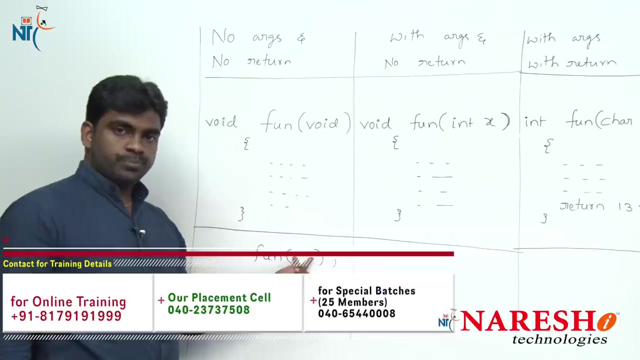 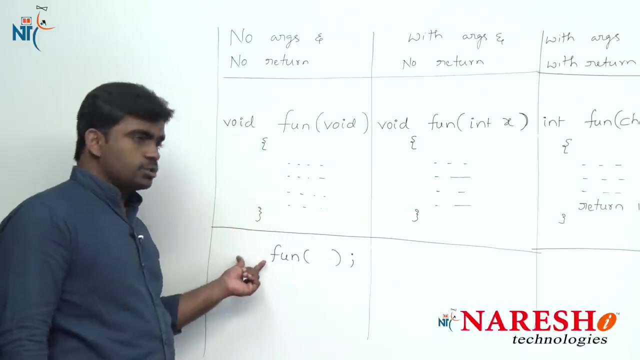 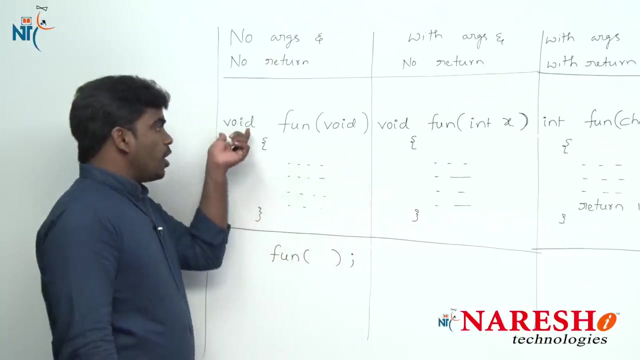 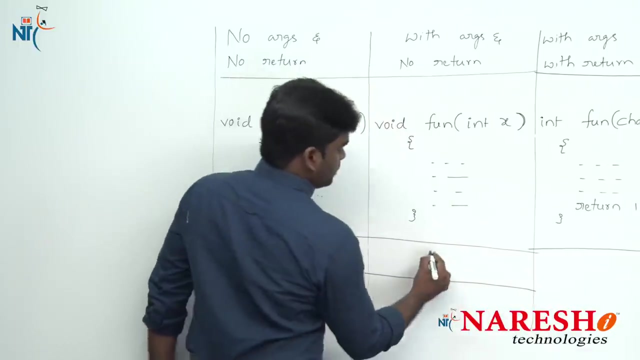 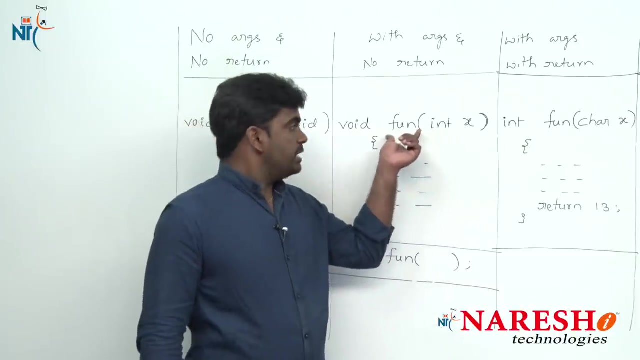 with no arguments and no return values. no means a void. we are writing no arguments, no return values. It is not giving anything, so no need to get. anything is a first one. and next come to that second one, function function. and now what it is expecting the function definition is: 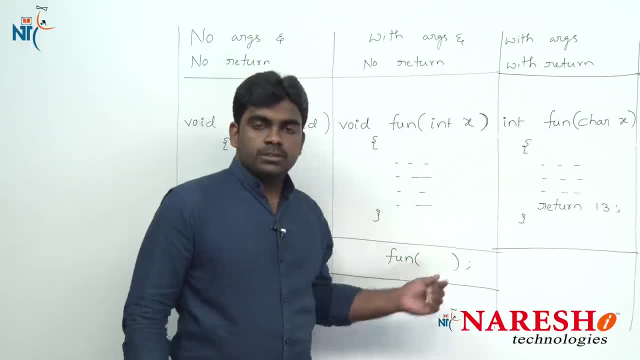 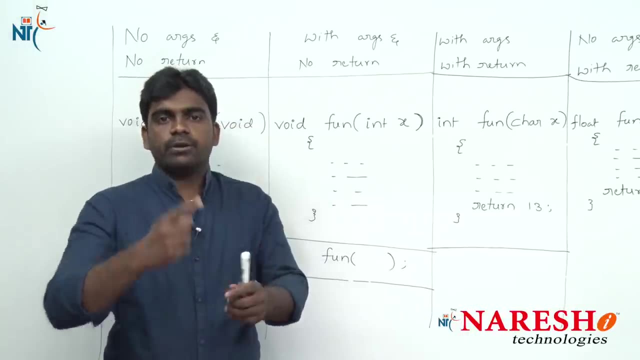 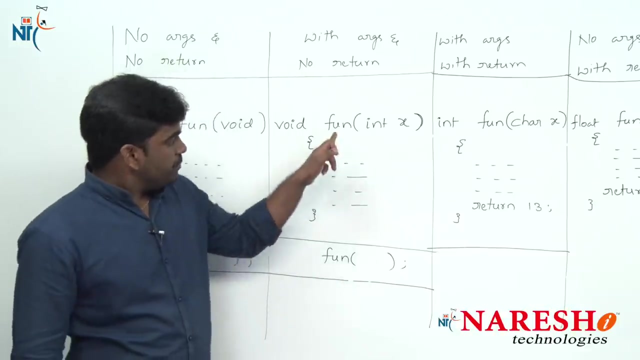 expecting an integer, So you have to pass integer. suppose, if you want to perform deposit operation, the bank personnel will expect some amount of money from you so that you have to pass, And only they can process that information. so here it is. whenever you call this function, 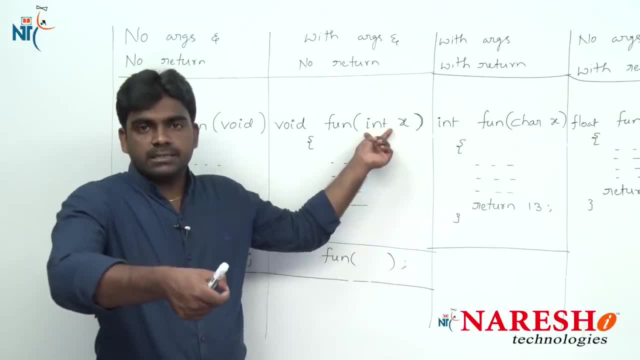 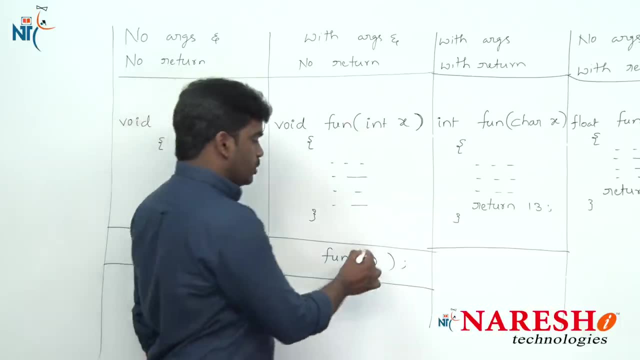 it is expecting integer, so you have to pass that integer. any integer you can pass, suppose simply 10. I am passing 10 is an integer, So that will go and store into x. now, x value 10. right then it will process the 10, but is 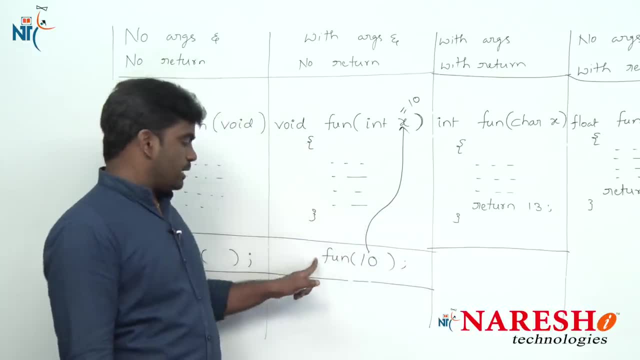 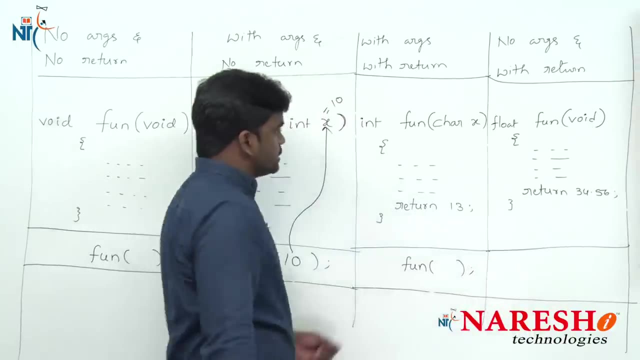 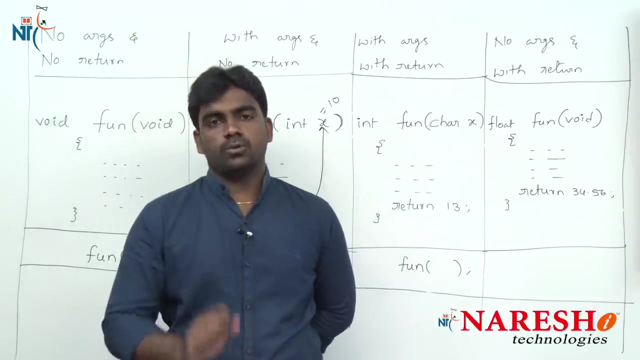 it giving anything? no, it is not giving anything, so no need to collect anything. and next come to the third one function. Now what it is expecting. it is expecting a character. in any programming language. we will represent characters using single quotes, right? So here it is. if you want to pass character, any character, you can pass a special symbol. 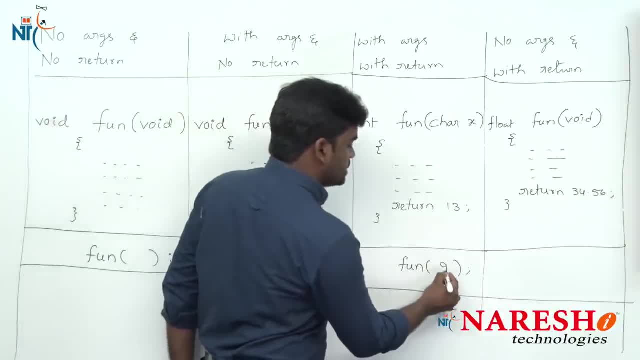 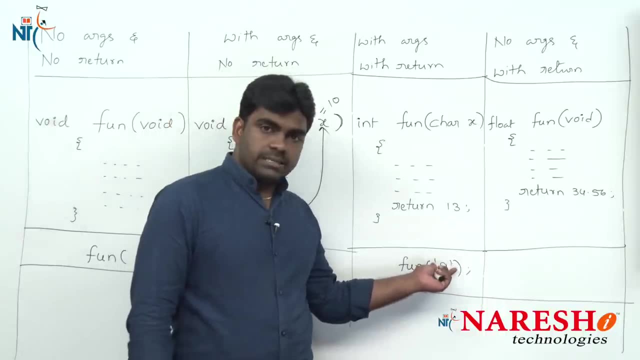 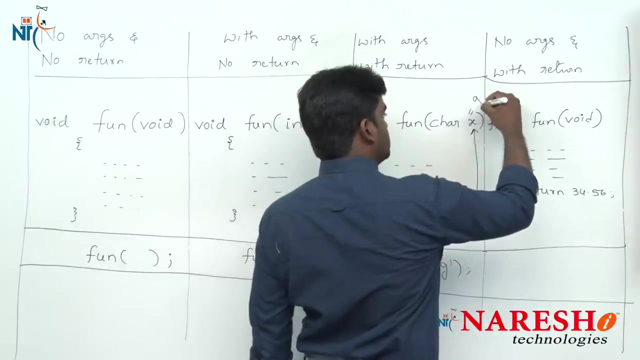 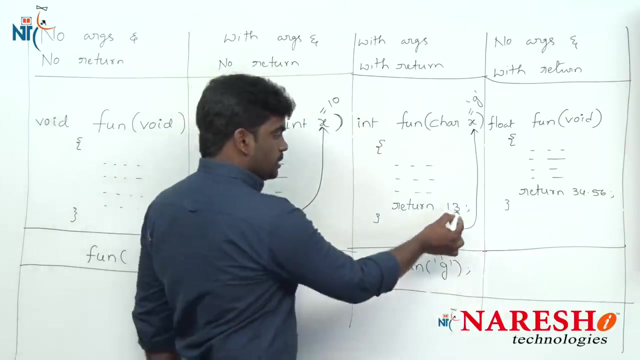 also you can pass, But we must place inside a single quotes. suppose g- I am passing right here it is, we are placing in a single quotes. whenever you call this function, that g will go and store into variable x. this is the value it will hold. input is over now. it is giving output. output 13. it is giving 13. we should collect. 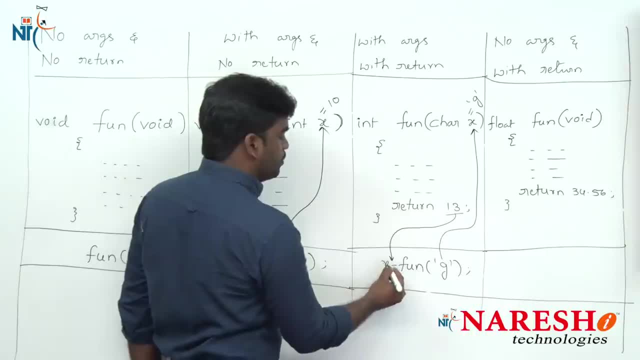 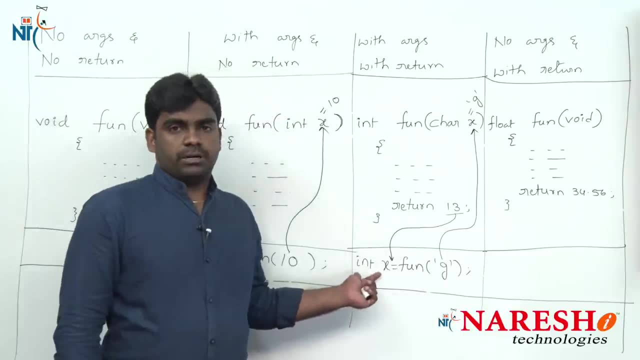 into another variable, or you can take a same variable also, no problem. but type is very, very important. what type it is returning is very, very important. right here it is returning 13. 13 is of type integer type. so we are collecting that result into integer type variable only for. 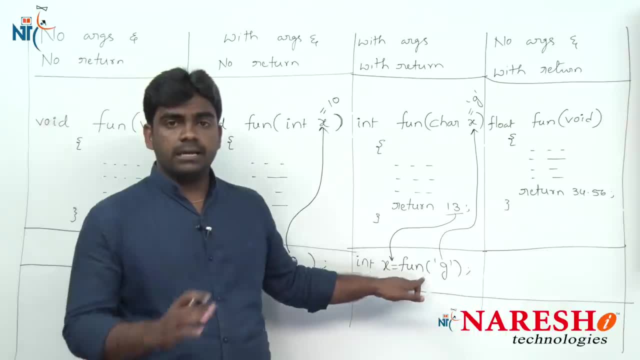 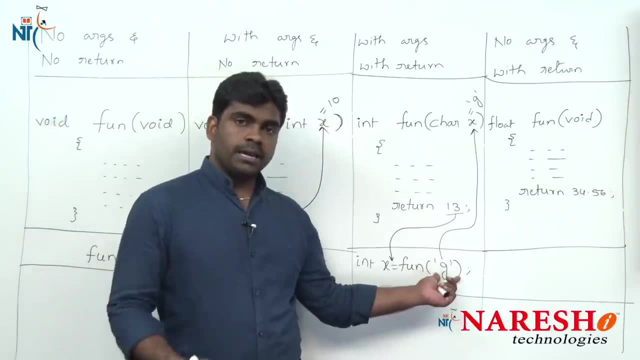 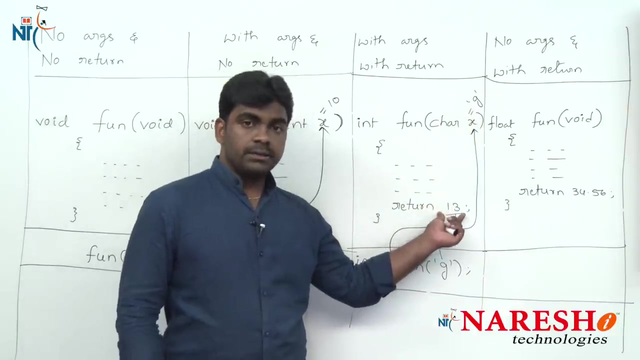 assignment operator: always right side data executes first. so right side data. we are calling the function and we are passing the input character. that character will go and store here and it is returning something. sir, what type it is returning? integer. it is returning that integer data we are collecting into x. x is of 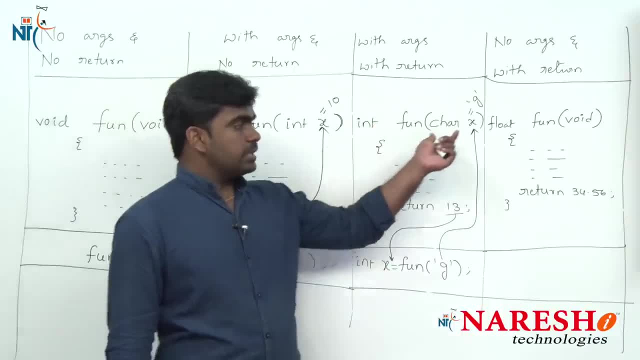 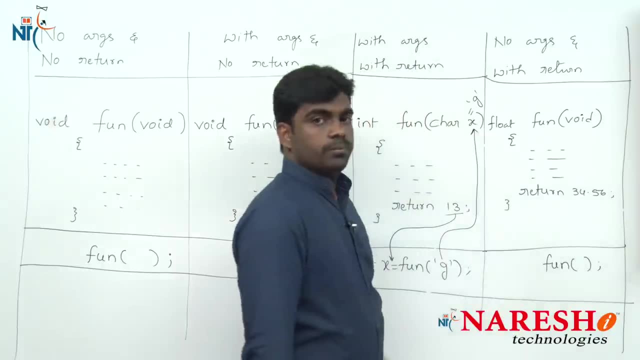 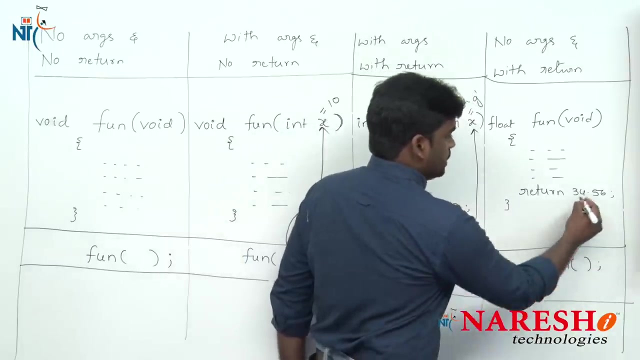 type integer, because return type is integer. and next the fourth classification. suppose here we are calling the function fun. is it expecting anything? no, type is a void type, so no need to pass anything to anyone. but here it is. we can expect something because it is returning a type.